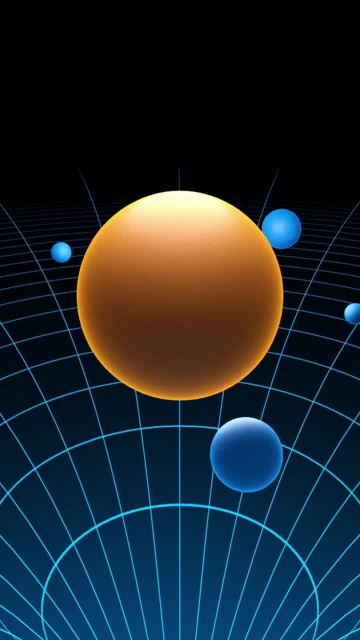 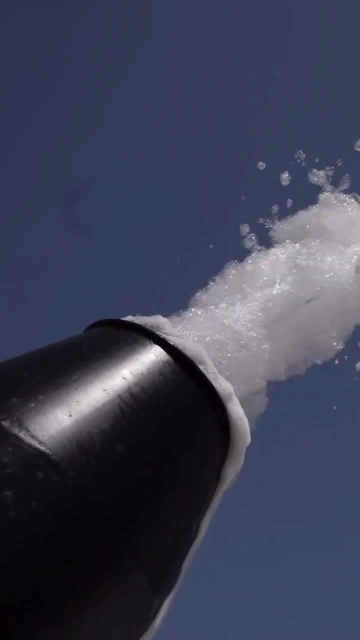 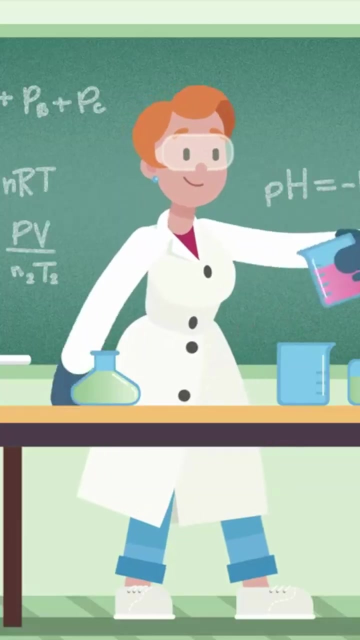 such as string theory, loop, quantum gravity and other cutting-edge models. One intriguing concept in quantum gravity is the idea of a quantum foam, a turbulent and fluctuating fabric of space and time at the tiniest scales. One of the major challenges. 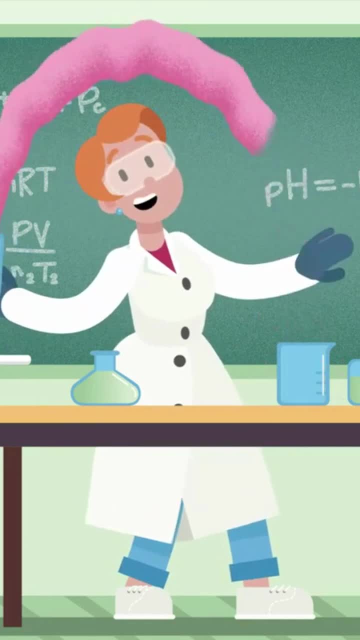 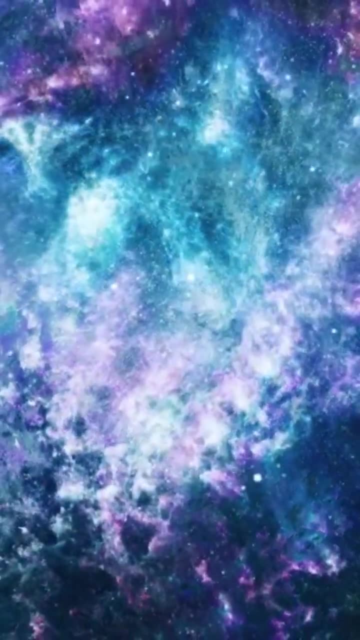 in quantum gravity is the extreme conditions at which gravity becomes quantum. Understanding these conditions can shed light on the behavior of particles and the structure of the universe. 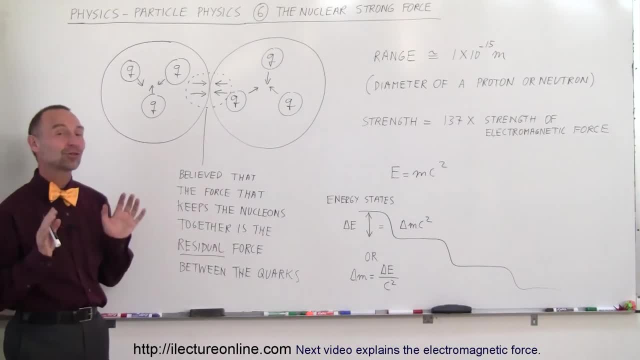 Welcome to our lecture online. Now we're going to talk about the nuclear strong force in a little bit more detail. So, jumping ahead, we did mention before that the nuclear strong force is responsible for keeping the quarks together that build the neutrons and the protons and all the other. 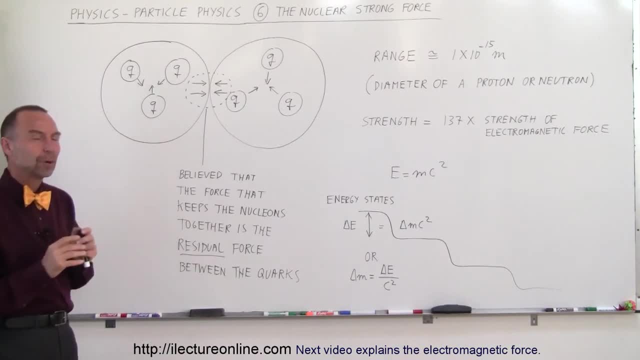 hadrons. Now we haven't had an overview yet of all those various particles. We will soon in the next several videos. But what we want to do first is take a look at the four forces of nature in a little bit more detail. So again, three quarks make up a proton, or three quarks make up 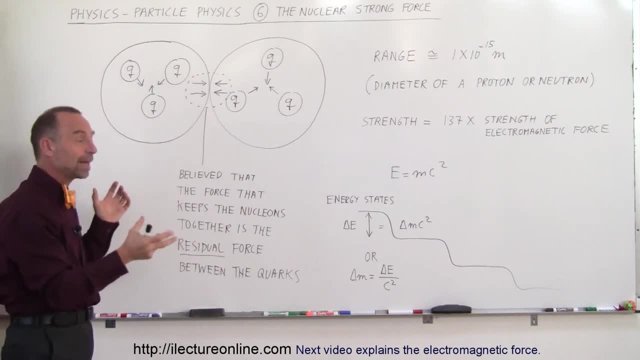 a neutron. There's a different combination of the quarks to make the various nuclear particles, such as neutrons and protons, And what we discovered was the nuclear strong force is responsible for keeping the quarks together. Now a very interesting note on that, and we'll talk about a little bit. 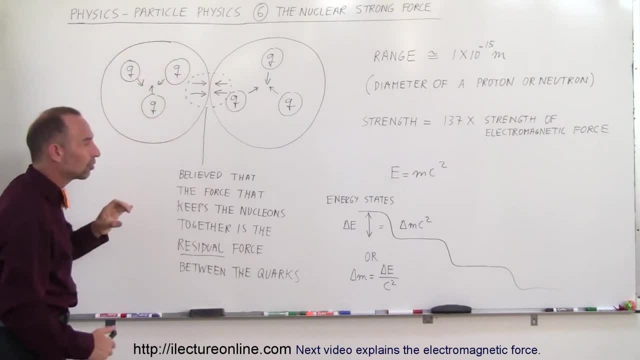 more detail later is that the mass of individual quarks is much, much smaller than the total mass of the nuclear strong force. So what we're going to do is take a look at the four forces of nature in a little bit more detail. So what we're going to do is take a look at the four forces of nature. 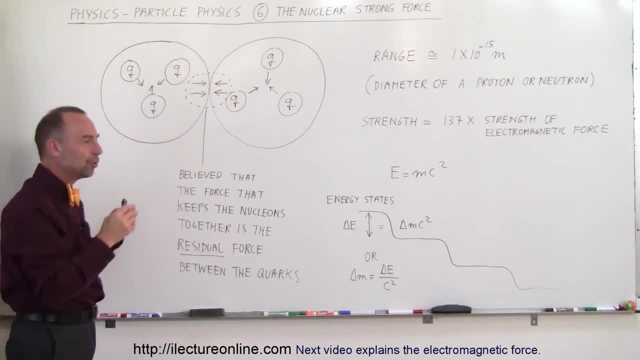 in a little bit more detail. So what we're going to do is take a look at the four forces of nature of the three quarks together forming a proton or neutron. If you were able to separate the quarks from one another in a separate matter- and we haven't been able to do that, we have not yet been.